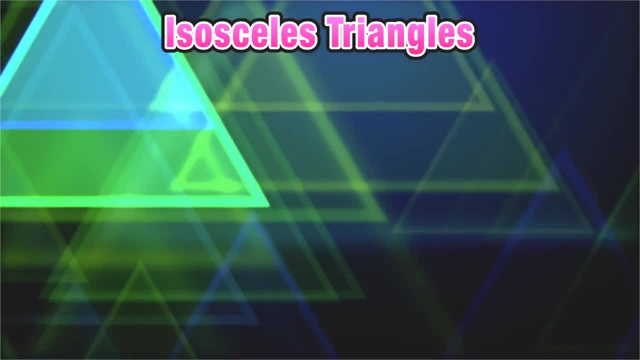 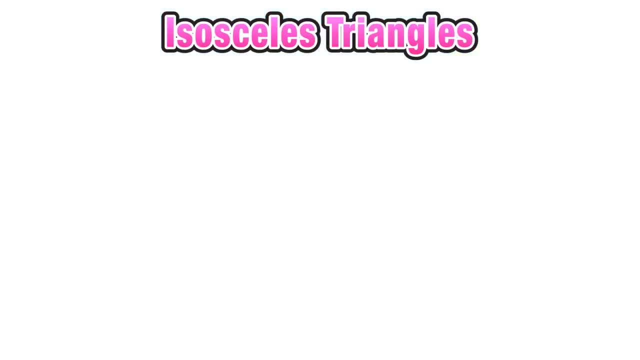 What's up again everyone. Thanks for joining me on this lesson. We're going to go ahead and explore the properties of isosceles triangles, So let's start out with a basic definition that says that a triangle with two congruent sides is called isosceles, And we can look. 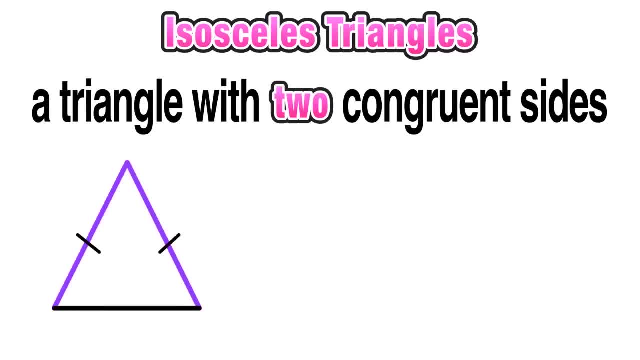 at some visual examples here, Notice that each of these three triangles has a pair of congruent sides, Which is denoted by those little slashed marks on the sides that are congruent to each other. And these are all examples of isosceles triangles. 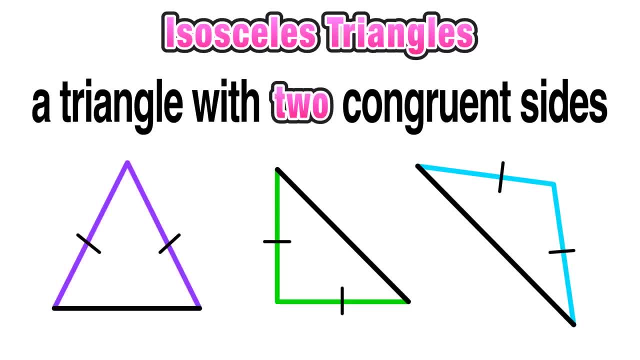 Let's take a look at some visual examples here. triangles: Their orientation may be different, that is, that they are all kind of rotated in a different way, but that actually does not make a difference here. So let's go ahead and take this. 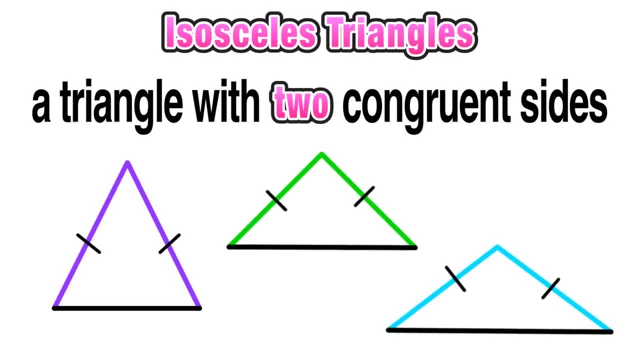 a step further. We're going to go ahead and spin around those two triangles so that all three of the isosceles triangles are facing the same way, with the congruent sides in the same spot. So now let's go ahead and just take a look at these isosceles triangles. 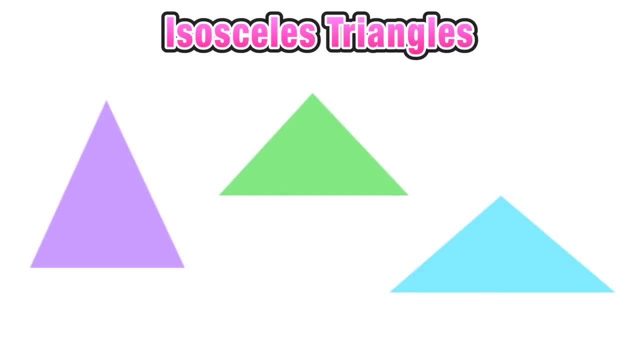 without any markings of angles or sides, And there's an important relationship that we want to see here. Imagine if we were to vertically cut these triangles in half, right down the middle. Our result would be a right triangle, just like the ones that are shown. 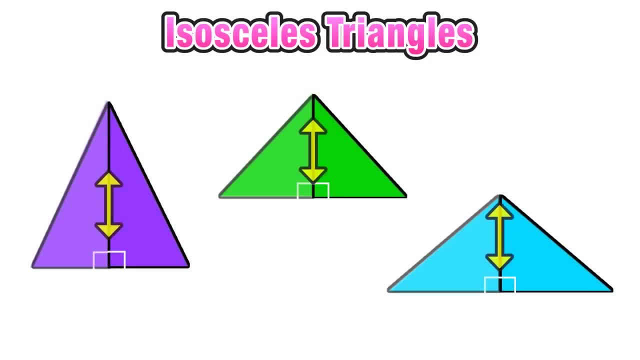 And if I take that right triangle and reflect it over that vertical line that we imagined cutting in half originally, our result would be the original isosceles triangles that we started with. Now we will revisit this relationship later on in the lesson, but for right now, 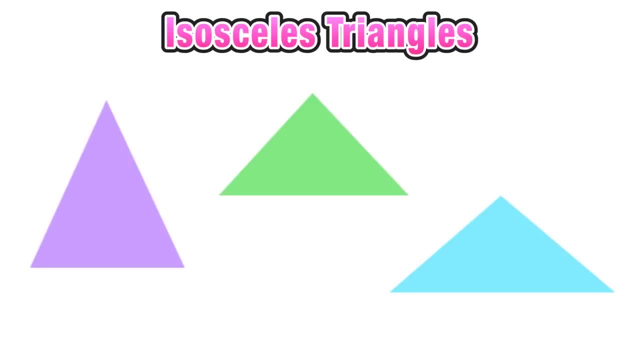 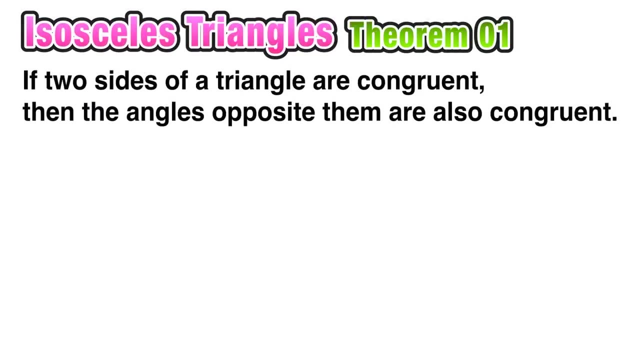 just keep this in mind as you're building the concept of exactly what an isosceles triangle is. Okay, so now we're ready for our first isosceles triangle theorem, which says that if two sides of a triangle are congruent, then the angles opposite them. 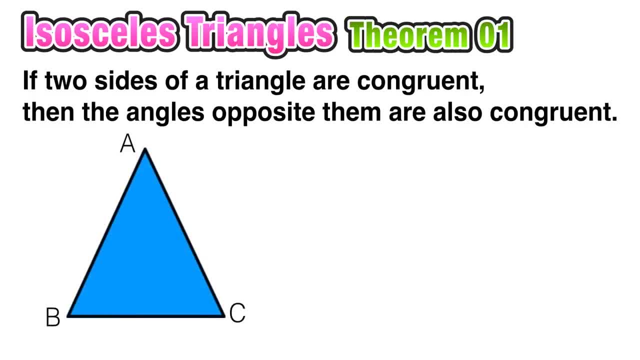 are also congruent. The first part of this theorem says that if two sides of a triangle are congruent, the angles opposite the sides of a triangle are congruent. So in this case we're going to say that if side AB is congruent to side AC, then the angles opposite of those sides are also congruent. 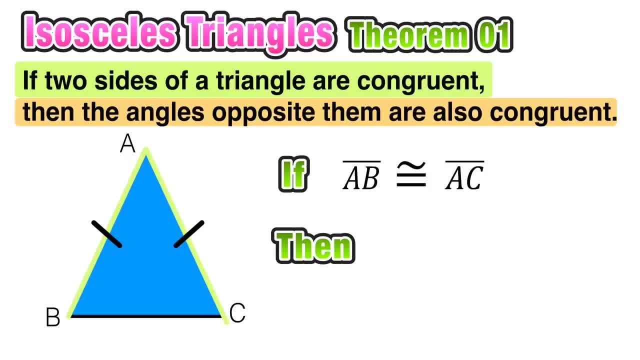 to each other. So let's visualize what that actually means. If we start at those two congruent sides and go opposite or across from them, we arrive at angles B and C And according to this theorem, angle B would be congruent to angle C, since they are opposite of sides that are congruent. 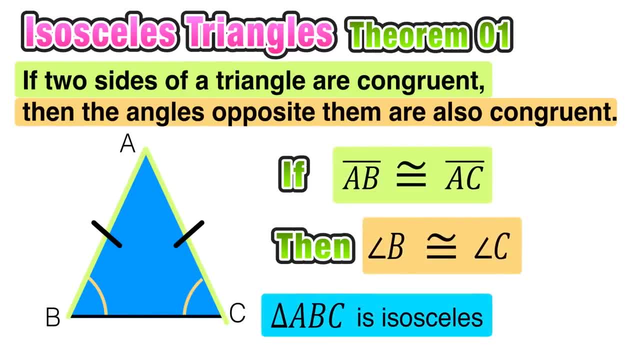 to each other. Now, obviously, triangle ABC is isosceles, And take a really good look at this image, because this is a classic representation of your typical isosceles triangle, where the two sides are congruent and the two angles- the base angles opposite those sides, are also congruent. 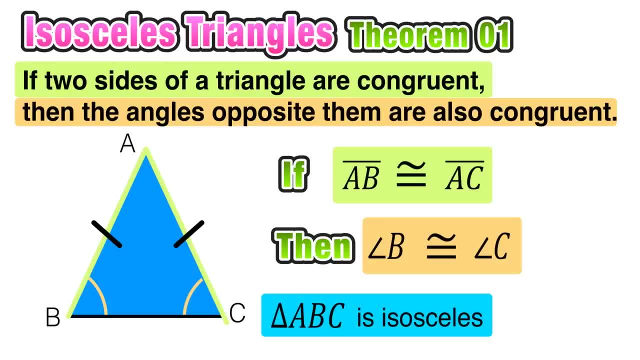 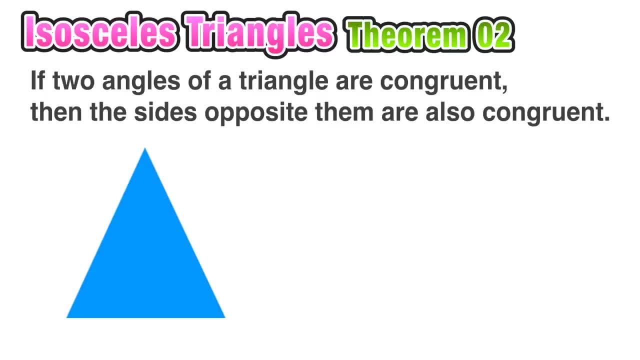 So keeping this relationship in mind will help us to better identify isosceles triangles in the future. So the isosceles triangle theorem that we are going to look at says that if two angles of a triangle are congruent, then the sides opposite them are also congruent, And this is kind of like. 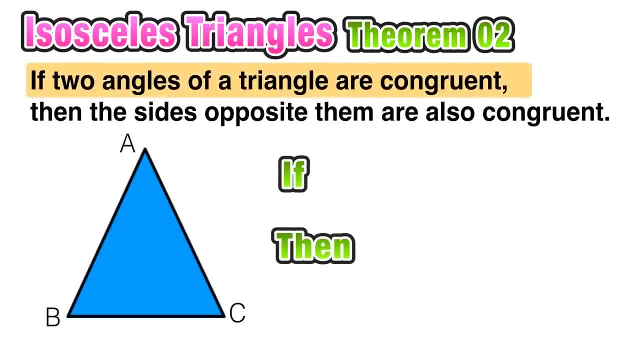 the reverse of the theorem that we just looked at. So again, if two angles of a triangle are congruent- in this case angle B is congruent to angle C- the base angles- then the sides that are opposite those angles are also congruent. So that would mean that side AB 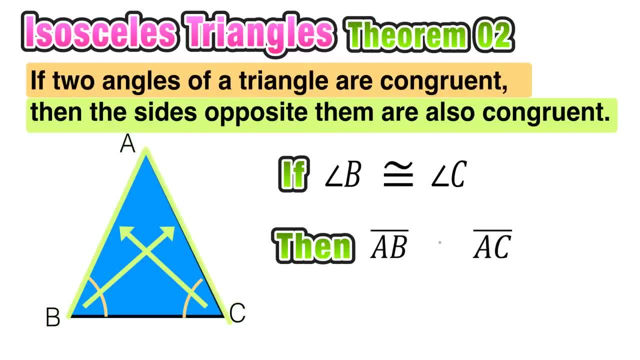 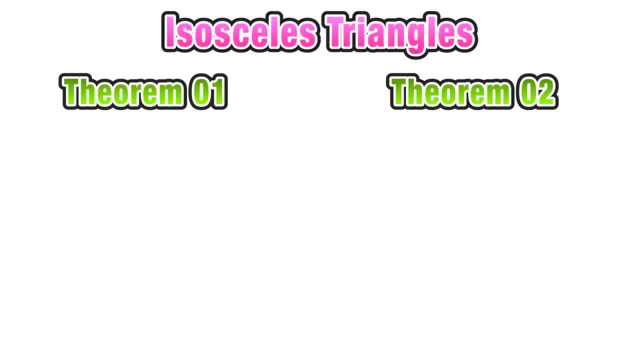 would have to be congruent to side AC, And that's pretty much how this theorem works. And again, because of this relationship, we can conclude that triangle ABC is isosceles. So we just looked at two important isosceles triangle theorems. Now let's quickly visually. 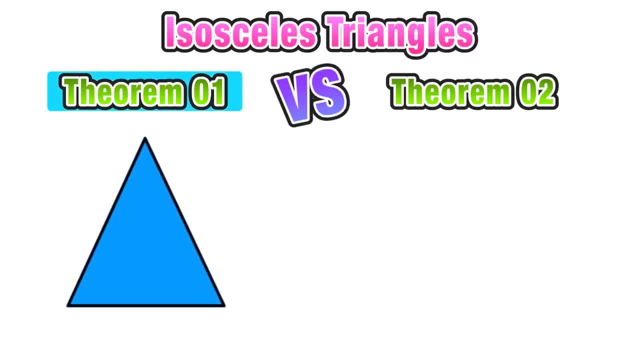 compare these two so we understand the difference between them. Theorem 1 said that if two sides in a triangle were congruent, then the sides opposite them are also congruent. So if two angles of a triangle are congruent, then the angles that were opposite from them were also congruent. Theorem 2 said that if two 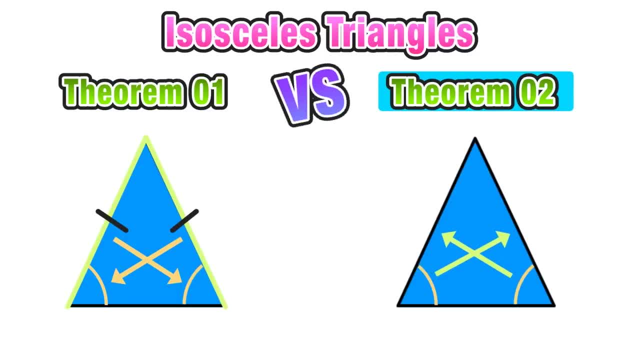 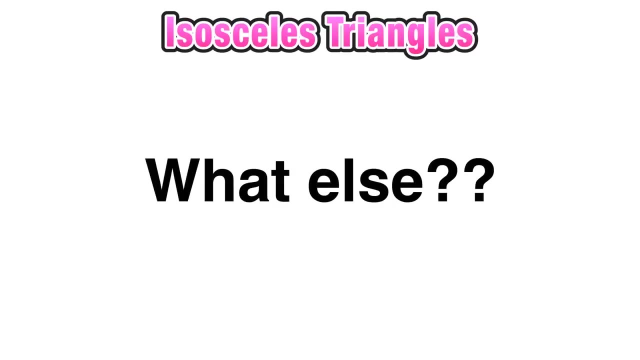 angles in a triangle were congruent, then the two sides opposite them are also congruent, So it's just like a reverse order between the two. And now that we're more comfortable with the basic definition and image of your typical isosceles triangle, let's look at what else that we should know about these kinds of triangles. 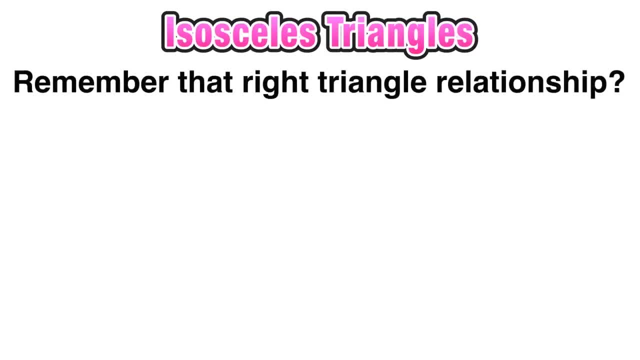 Ans. now that we're more comfortable with the basic definition and image of your typical isosceles triangle, let's look at what else we should know about these kinds of triangles, that we should know about these kinds of triangles. So this is where we're going to go back to that. 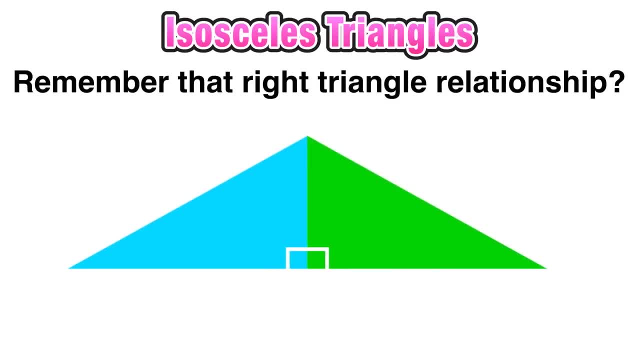 right triangle relationship that we explored earlier, where we looked at an isosceles triangle as two congruent right triangles that were kind of back to back or reflected over a vertical line. Now, since those triangles are congruent, we know that corresponding angles and corresponding sides 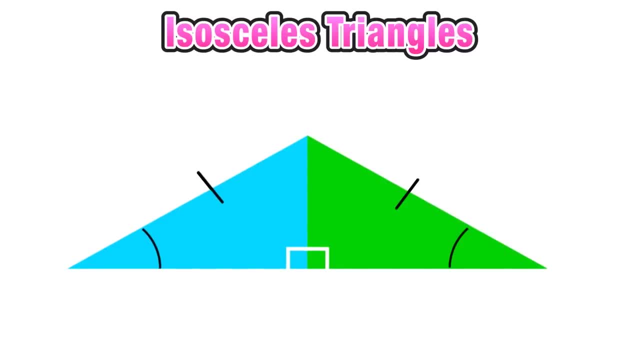 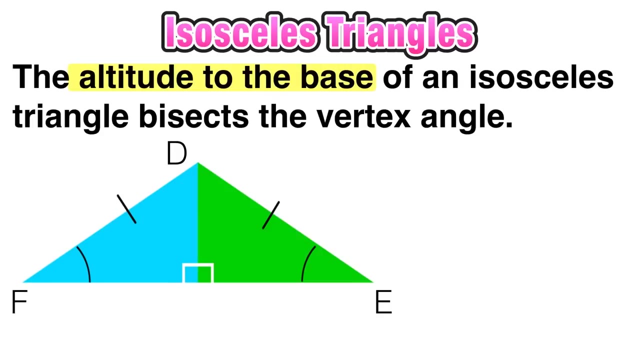 will also be congruent, And we see here that this matches our definition of an isosceles triangle. Now, with this in mind, we can take this one step further and say that the altitude to the base of an isosceles triangle bisects the vertex angle. So let's now visualize what this means. If we 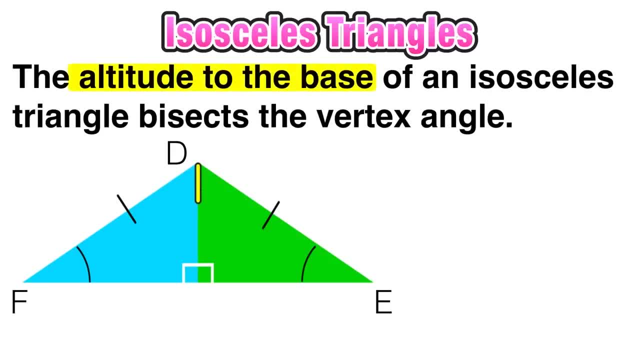 call this triangle, triangle DEF, and we draw that altitude from angle D to the base of the triangle. okay, we make a new point, called a triangle DEF, and we draw that altitude from angle D to the base angle. okay, So we can say that this angle is cut into two congruent halves. 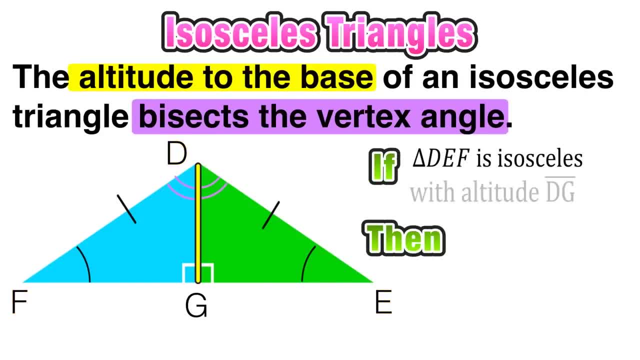 So if triangle DEF is isosceles with altitude DG, then our conclusion is that angle FDG is congruent to angle EDG, again, because that's the angle that we want to draw. So if triangle DEF is isosceles with altitude DG, 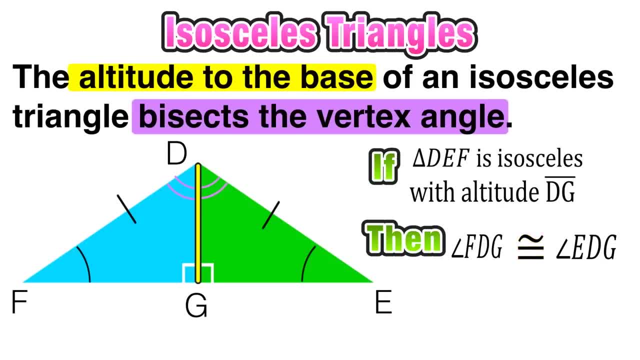 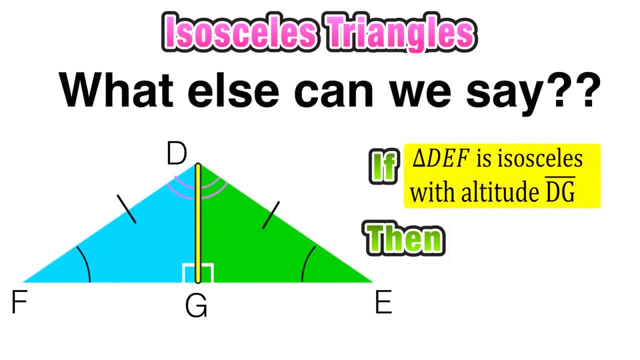 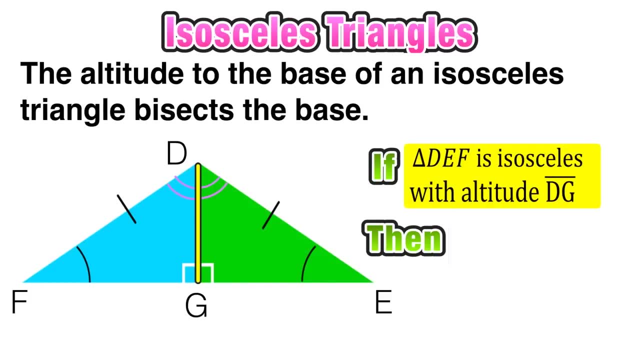 then our conclusion is that angle FDG is congruent to angle EDG. altitude bisects the vertex angle into two congruent pieces. Now is there anything else that we can say about isosceles triangles by using these relationships? Now it turns out that that altitude DG does more than just bisect. 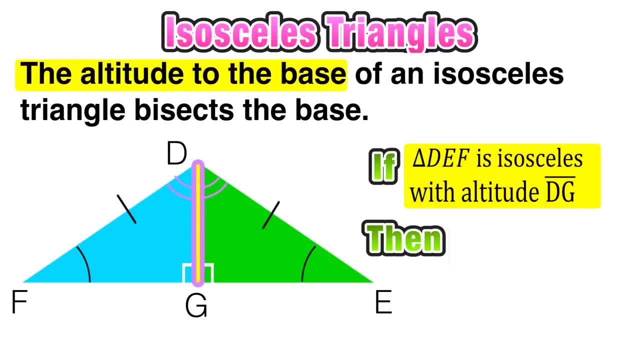 the vertex angle it also bisects the base. So again that line DG will cut the base, that big line FE, again into two congruent halves And we can conclude that FG would be congruent to EG based on this relationship And again, if we